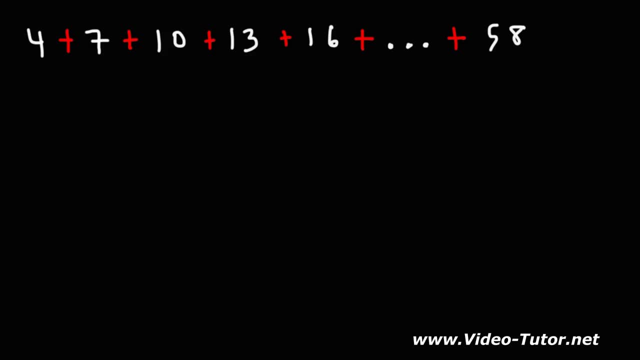 But we're going to use a formula to get the answer. Now, here is the formula we need to calculate the sum of an arithmetic series. It's going to be the first term, a sub 1, plus the last term, a sub n, divided by 2.. 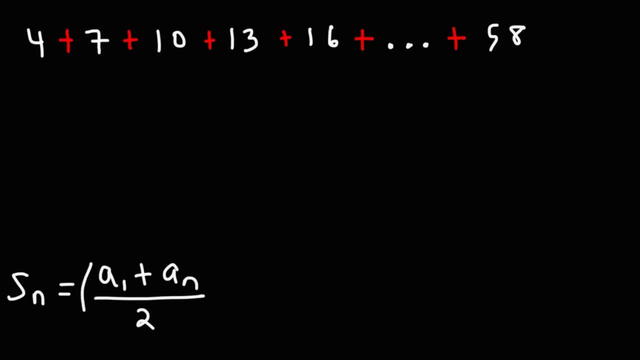 So it's the average of the first and last terms multiplied by the number of terms. Now we know the value of the first term: It's a sub 1,, that's 4.. The last term, a sub n, is 58.. 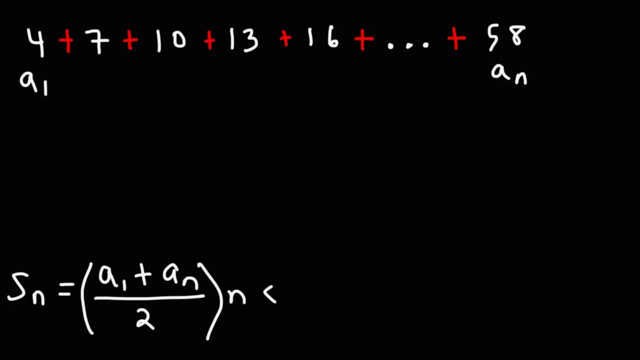 What we don't know in this problem is the number of terms n. So that's what we've got to find, And we could use this formula to get the value of n. a sub n is equal to a sub 1 plus n minus 1 times d. 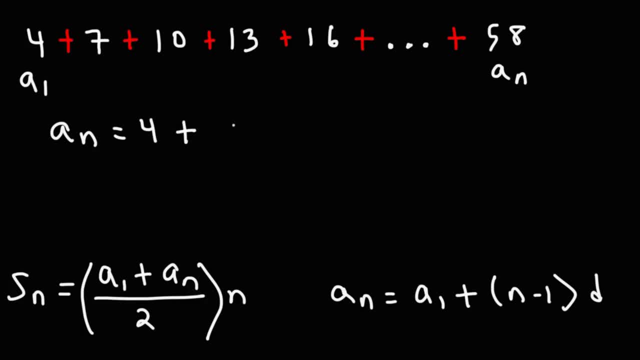 Now we know what a sub 1 is. The first term is 4.. We don't know the value of n. d is the common difference. To go from 4 to 7, we need to add 3.. And to go from 7 to 10, we need to add 3.. 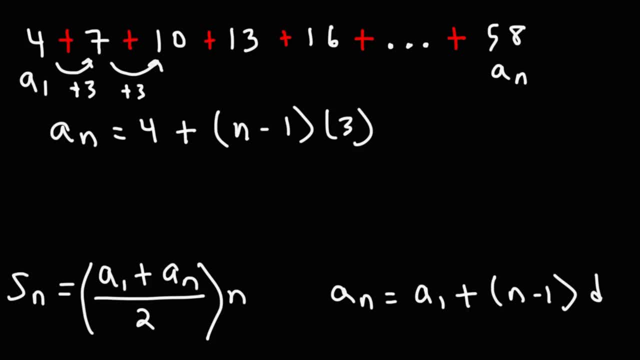 So the common difference is 3.. Now we already know the value of a sub n. a sub n is 58. So we have: 58 is equal to 4 plus. I'm going to distribute the 3 to the n minus 1.. 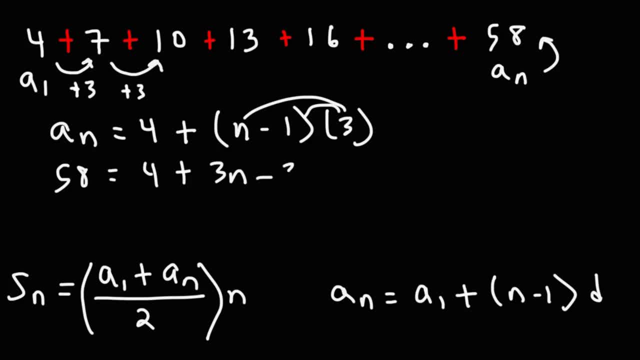 So this becomes 3n minus 3.. Combining like terms we have 4 minus 3,, which is positive 1. So 58 is equal to 4.. 58 is equal to 3n plus 1. Subtracting both sides by 1, we get 57 is equal to 3n. 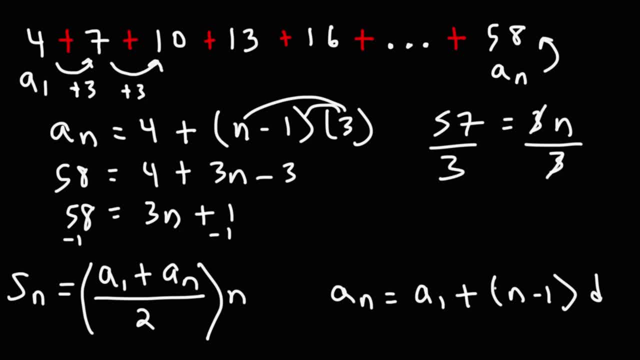 Dividing both sides by 3, we get n is equal to 19.. So this is the first term. The last term is the 19th term. So we're looking for the sum of the first 19 numbers in this series. 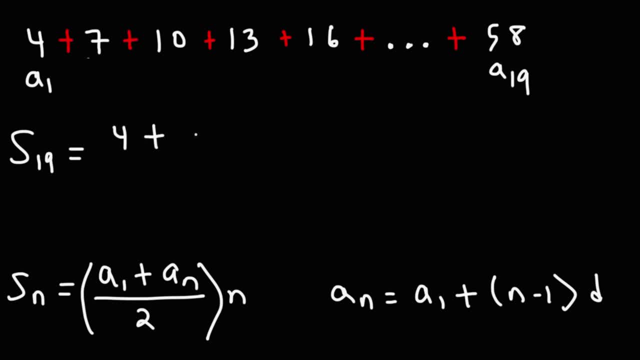 a sub 1,. the first term is 4.. a 19,. the last term is 58,. divided by 2, times 19, terms 4 plus 58, is 62.. 62 divided by 2 is 31.. 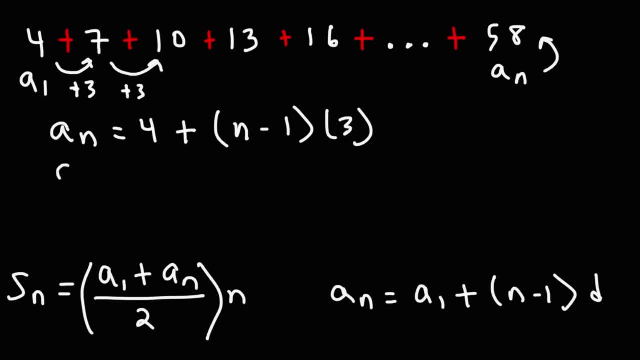 Now, we already know the value of a sub n. a sub n is 58. So we have 58 is equal to 4 plus... I'm going to distribute the 3 to the n minus 1. 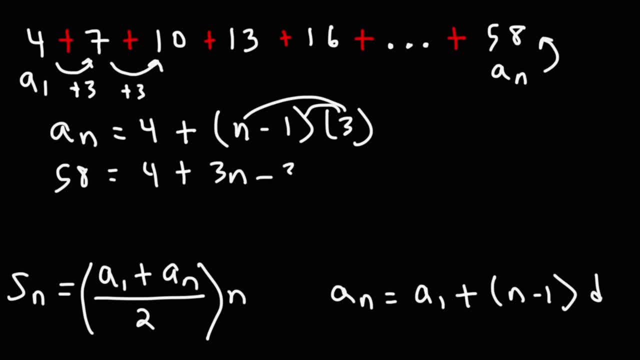 So this becomes 3n minus 3. Combining like terms, we have 4 minus 3, which is positive 1. 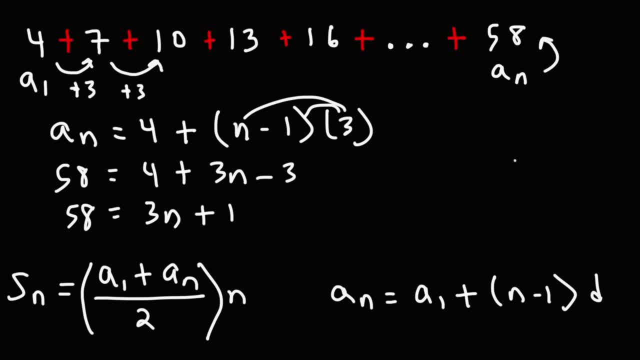 So 58 is equal to 4. 58 is equal to 3n plus 1. Subtracting both sides by 1, we get 57 is equal to 3n. 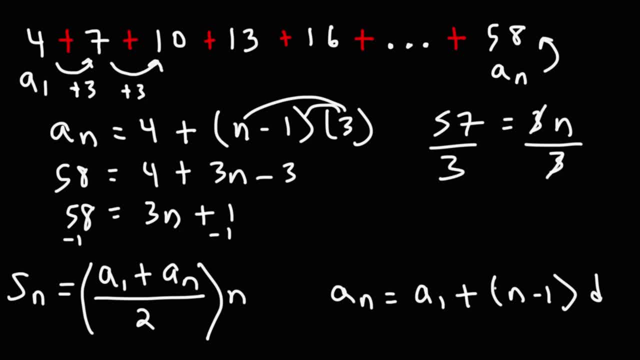 Dividing both sides by 3, we get n is equal to 19. So this is the first term. The last term is the 19th term. So we're looking for the sum of the first 19 numbers in this series. 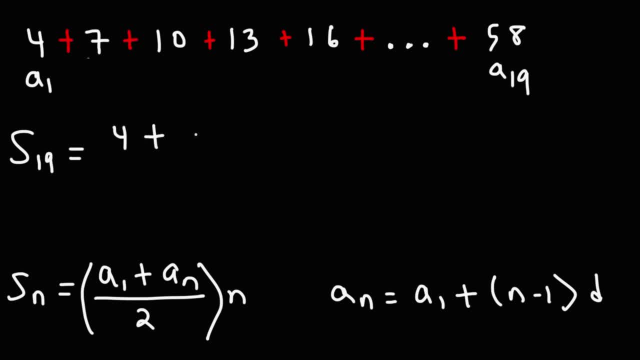 a sub 1, the first term is 4. a 19, the last term is 58, divided by 2, times 19 terms. 4 plus 58 is 62. 62 divided by 2 is 31. So the average of these two numbers is 31. 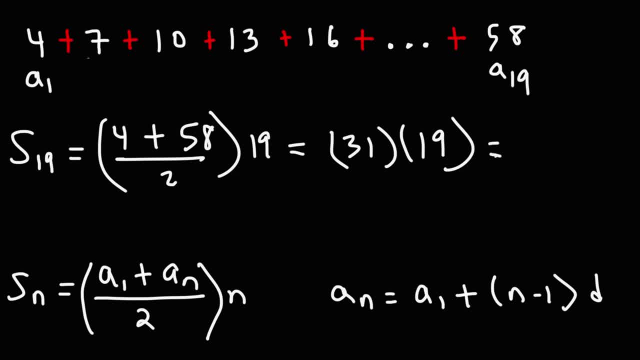 So we take the average, multiply it by the number of terms, and that's going to give us the sum of the arithmetic series. And that's going to be 589. 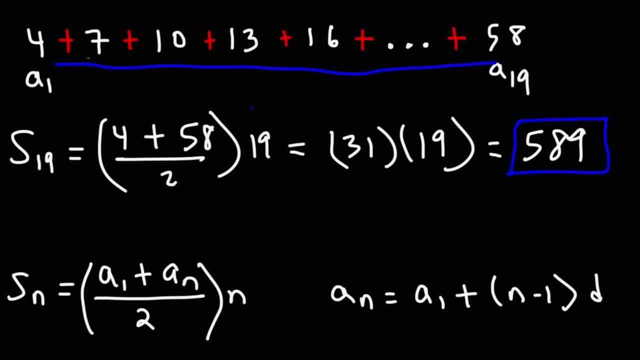 So if you were to write out all the numbers from 4 to 58, going up by 3, and if you add those numbers, you should get this answer, 589. 589. 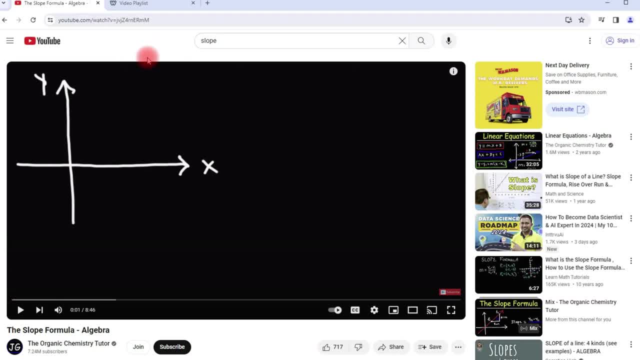 By the way, for those of you who want access to more video-related content, feel free to check out the links in the description. 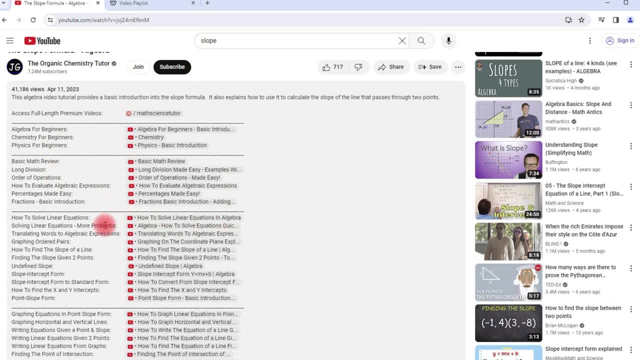 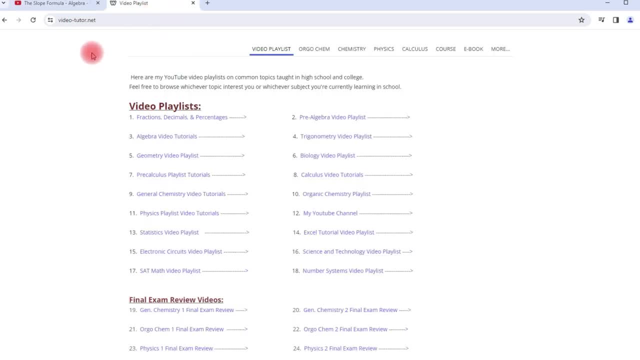 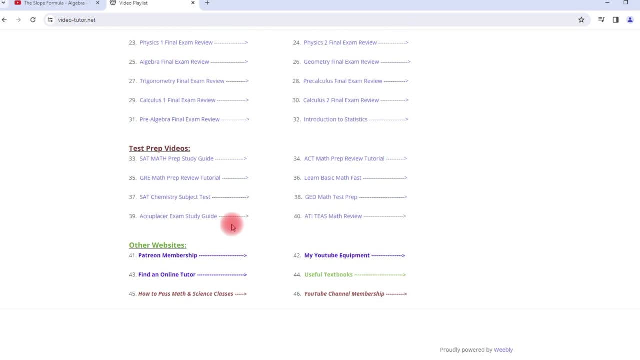 If you click on this more button, you're going to see other videos relating to the video that you're currently watching. And these links are separated by chapter. And of course, you could check out my website, video-tutor.net, where you'll get access to my video playlists, final exam videos, and also test prep videos. So feel free to take a look at that when you get a chance. 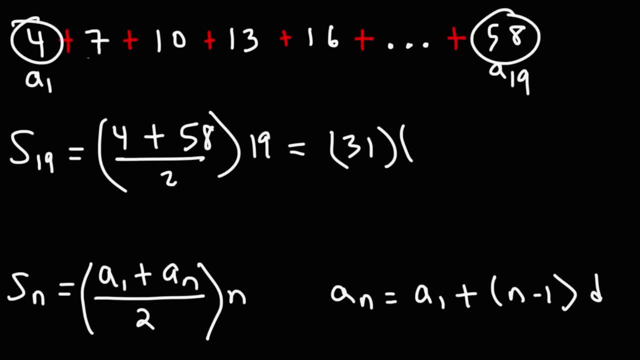 So the average of these two numbers is 31.. So we take the average, multiply it by the number of terms, and that's going to give us the sum of the arithmetic series, And that's going to be 589.. So if you were to write out all the numbers from 4 to 58,, 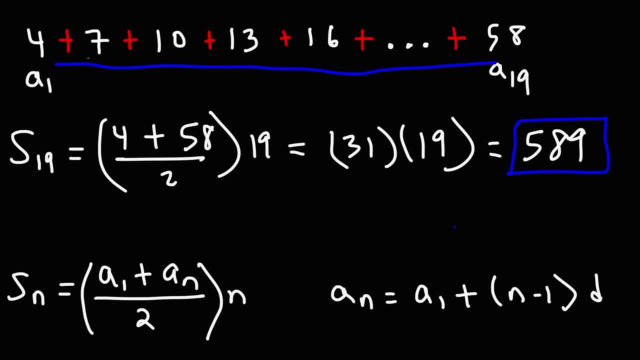 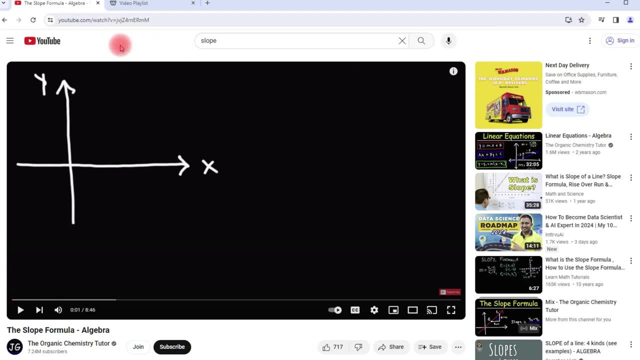 going up by 3, and if you add those numbers, you should get this answer: 589.. 589.. By the way, for those of you who want access to more video-related content, feel free to check out the links in the description. 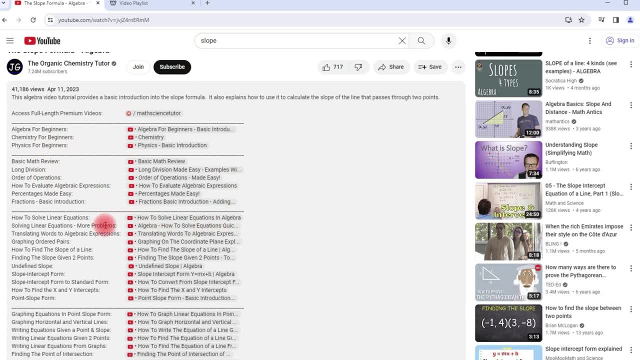 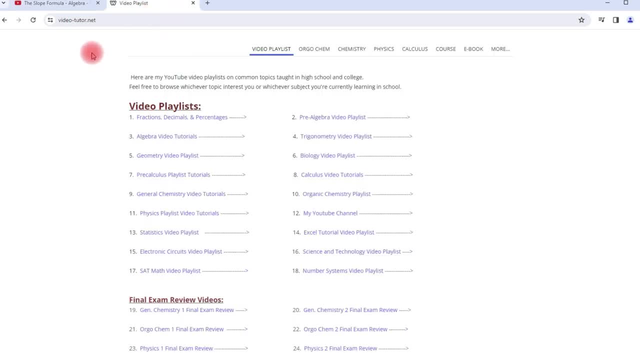 If you click on this more button, you're going to see other videos relating to the video that you're currently watching, And these links are separated by chapter. And, of course, you could check out my website, video-tutornet, where you'll get access to my video playlists. 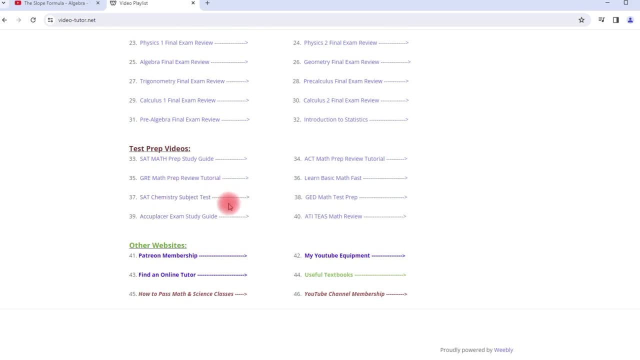 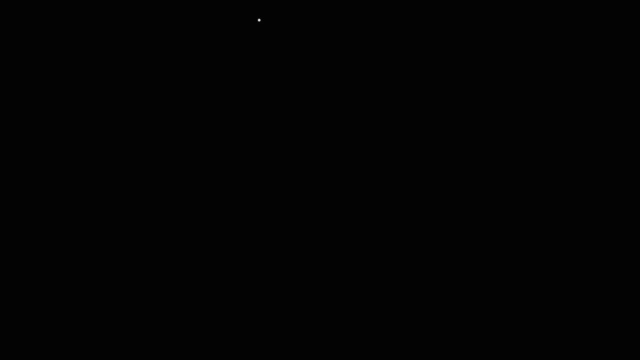 final exam videos and also test prep videos, So feel free to take a look at that when you get a chance. Now let's work on another problem. So let's say we have the following arithmetic series: So this time it's going in decreasing order. 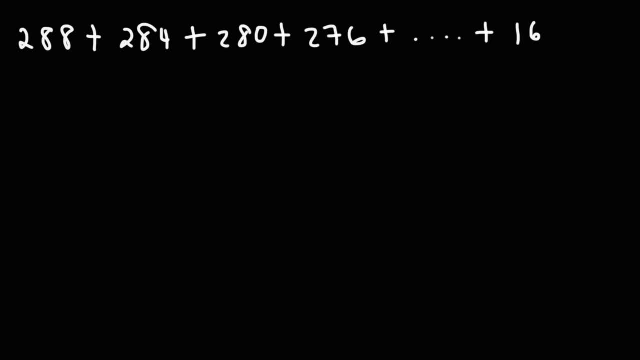 So what's the sum of this series? From 288 to 16, with each successive term decreasing by 4.. Feel free to pause the video if you want to try this Now. we know. the first term is 288.. The last term is 16.. 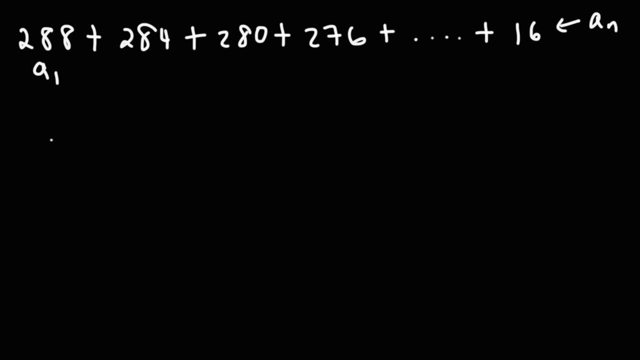 Just like before, we need to calculate the value of n, And so we could use this formula to do that: a sub n is 16.. a sub 1 is 288.. And d, the common difference as we go from a to b. 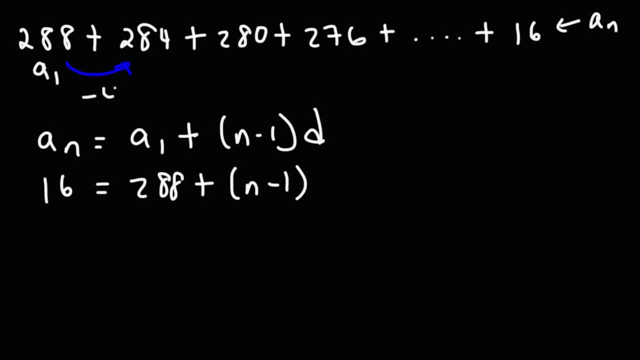 from the first to the second term, we need to add 4.. I mean negative 4.. And going from the second to the third term, we need to add negative 4.. So the common difference is not positive 4, but negative 4.. 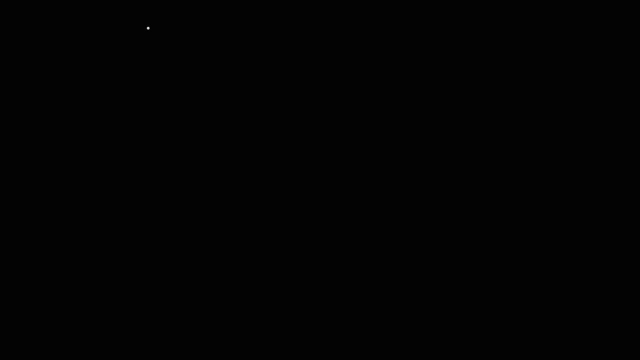 Now, let's work on another problem. So let's say we have the following arithmetic series. So this time, it's going in decreasing order. 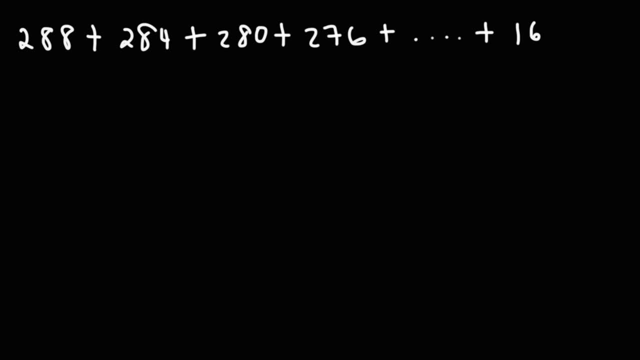 So what's the sum of this series? From 288 to 16, with each successive term decreasing by 4. Feel free to pause the video if you want to try this. 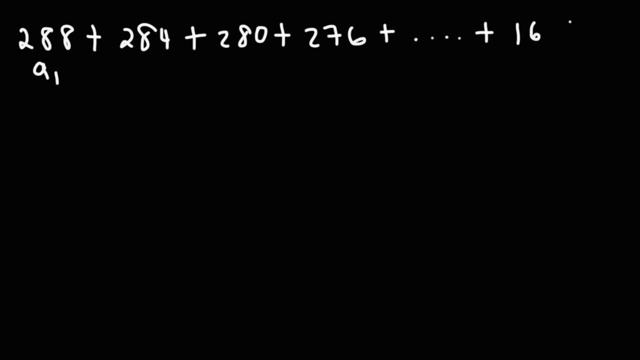 Now, we know the first term is 288. The last term is 16. Just like before, we need to calculate the value of n. And so we could use this formula to do that. a sub n is 16. a sub 1 is 288. 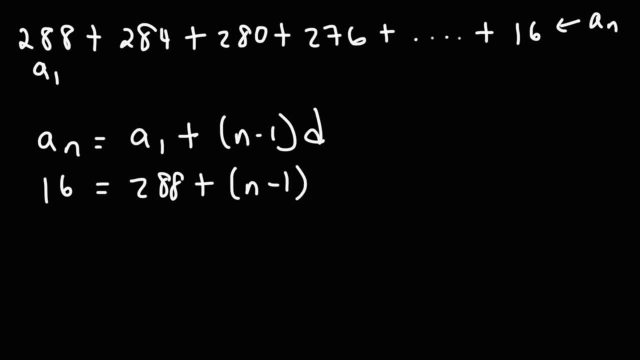 And d, the common difference, as we go from a to b, from the first to the second term, we need to add 4. I mean, negative 4. And going from the second to the third term, we need to add negative 4. So the common difference is not positive 4, but negative 4. 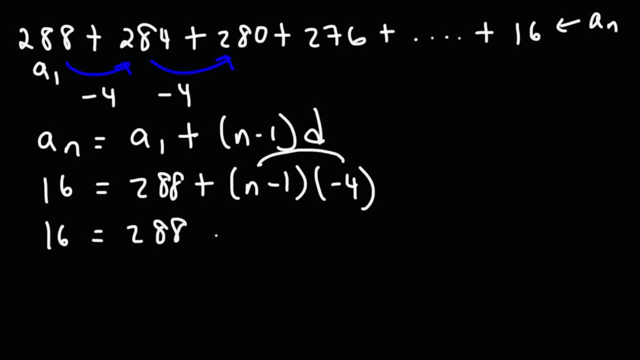 So what I'm going to do now is distribute the negative 4 to n minus 1. So we're going to have negative 4n plus 4. 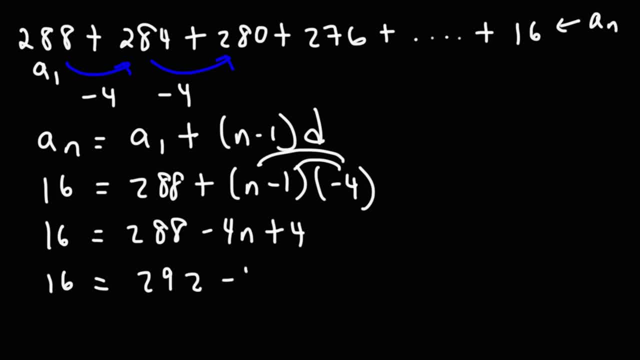 Now, 288 plus 4 is 292. Now, 288 plus 4 is 292. 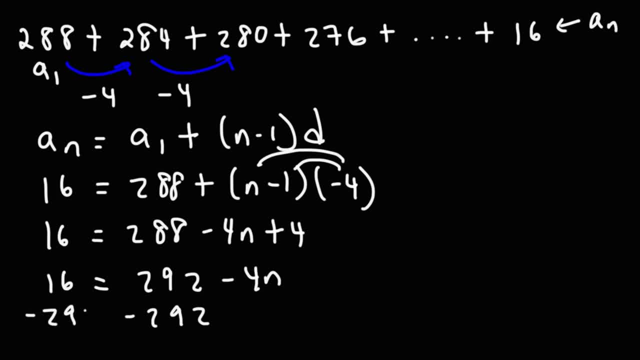 Next, I'm going to subtract both sides by 292. 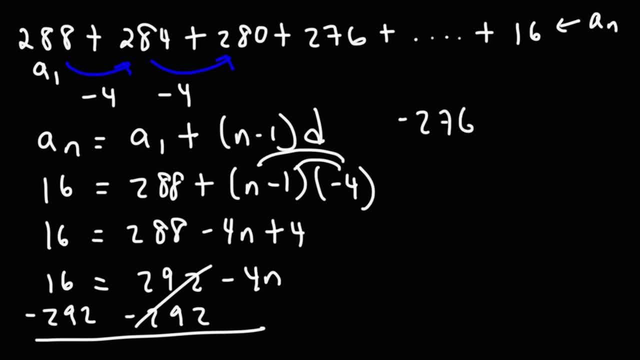 16 minus 292 is negative 276. And that's equal to negative 4n. 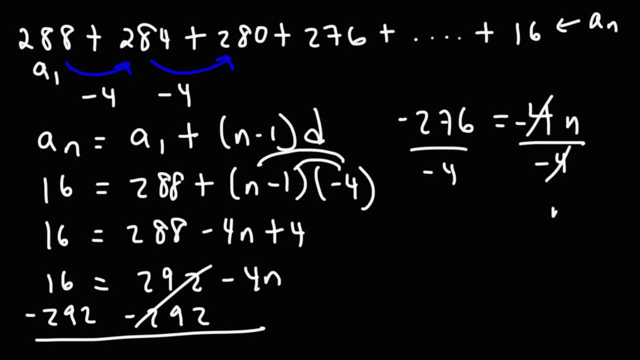 So dividing both sides by negative 4 will give us the value of n. 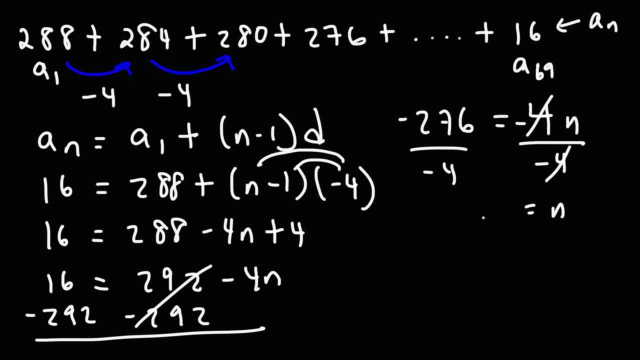 And n is 69. So this is the 69th term. 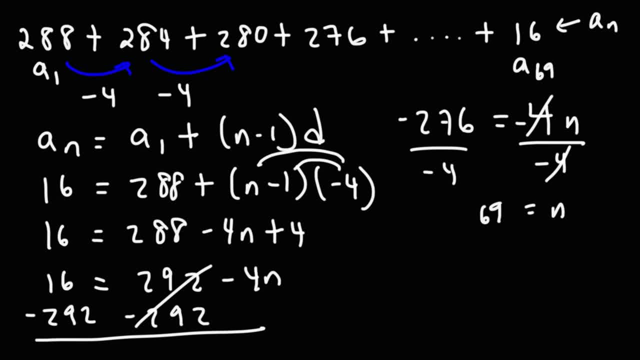 And we'll do this again. Also, I'm going to divide by 2, which will give us 169. So this will give us the value of 2n. And we're going to divide this by 3n. 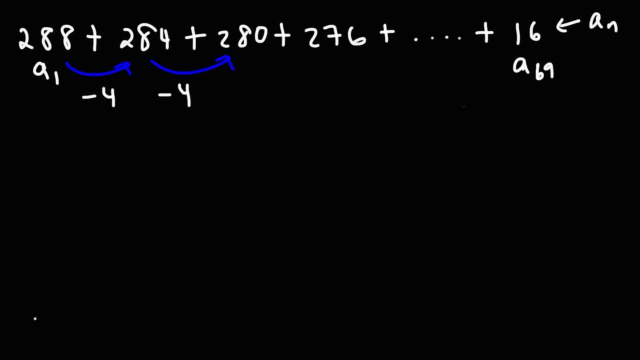 So now that we know how many terms are in the sequence, we can now calculate the sum using this formula. So it's going to be the first term plus the last term divided by 2 times the number of terms. 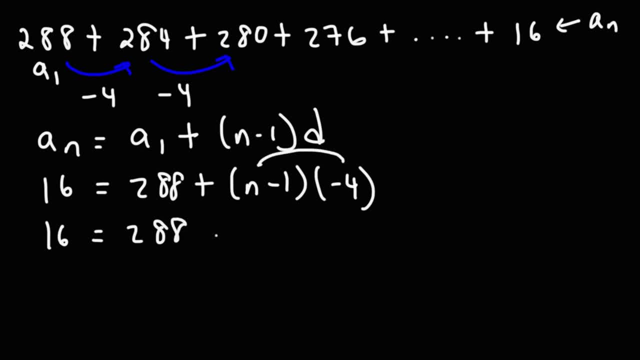 So what I'm going to do now is distribute the negative 4 to n minus 1.. So we're going to have negative 4n plus 4.. Now 288 plus 4 is 292.. Now 288 plus 4 is 292.. 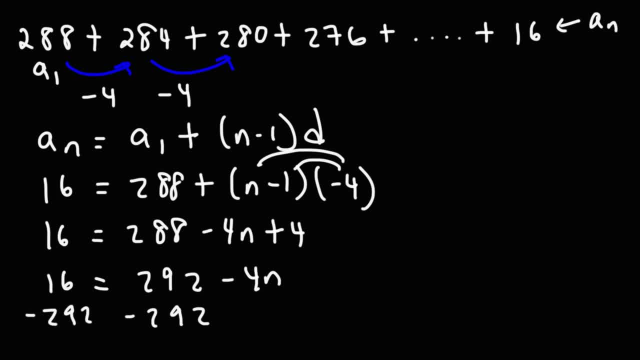 So I'm going to subtract both sides by 292.. 16 minus 292 is negative 276.. And that's equal to negative 4n. So dividing both sides by negative 4 will give us the value of n, And n is 69. 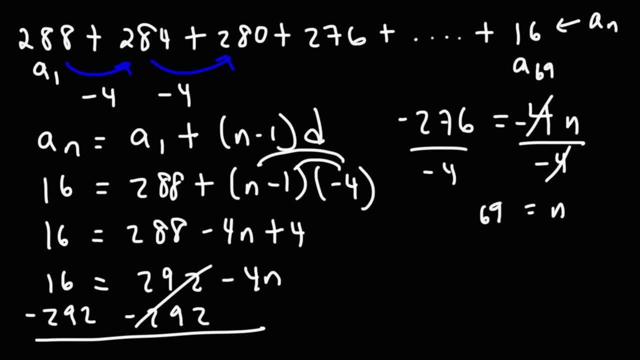 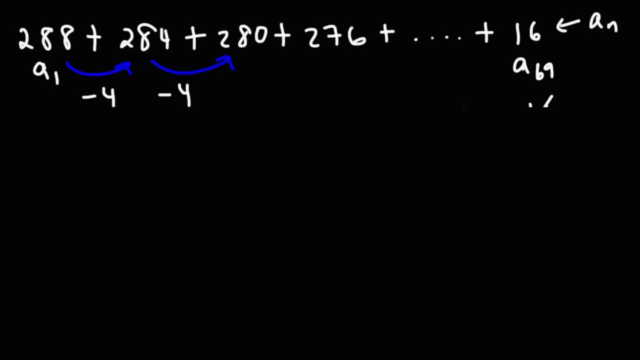 So this is the 69th term. so now that we know how many terms are in the sequence, we can now calculate the sum using this formula. so it's going to be the first term plus the last term, divided by two times the number of terms. so we want to find the sum of. 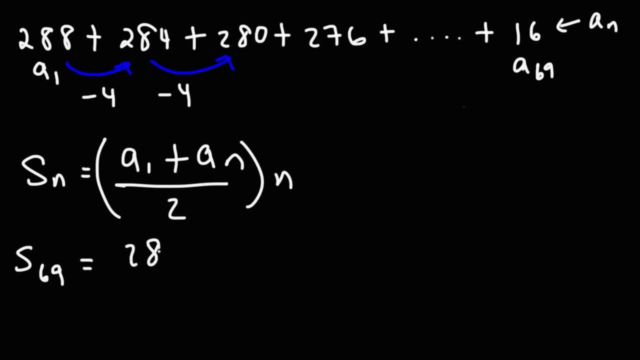 the first 69 terms. the first term is 288, the 69th term is 16 and n is 69. now 288 plus 16, that's 304. 304 divided by 2 tells us that the average of all the numbers in this sequence is going to be 152. 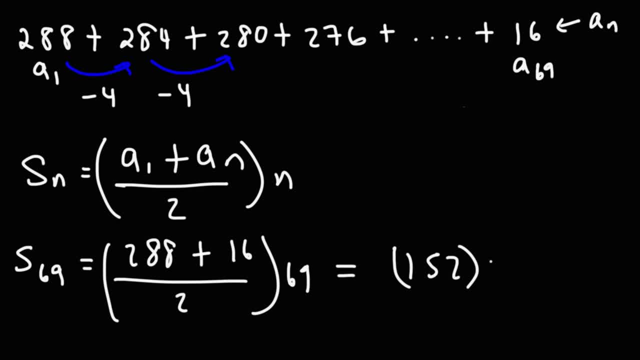 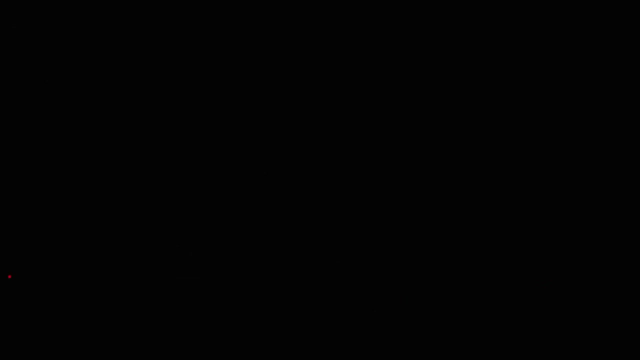 so, which is the average of the first and last term. so 152 times 69 is 10 488, and so that's how you can calculate the sum of this arithmetic series. for the sake of practice, i'll give you another one. so let's say we have the number. 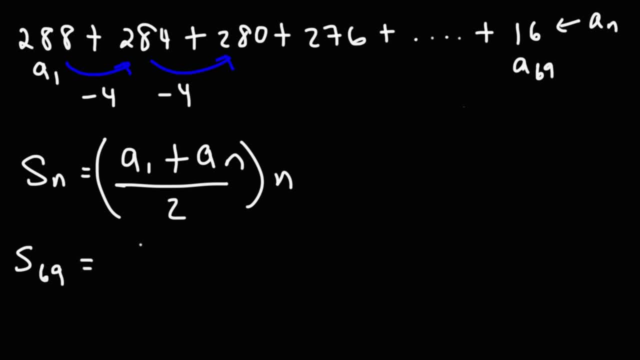 So we want to find the sum of the first 69 terms divided by two, times the number of terms. 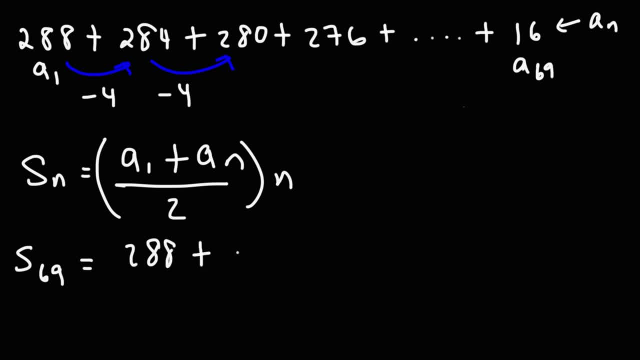 first term is 288, the 69th term is 16, and n is 69. Now 288 plus 16, that's 304. 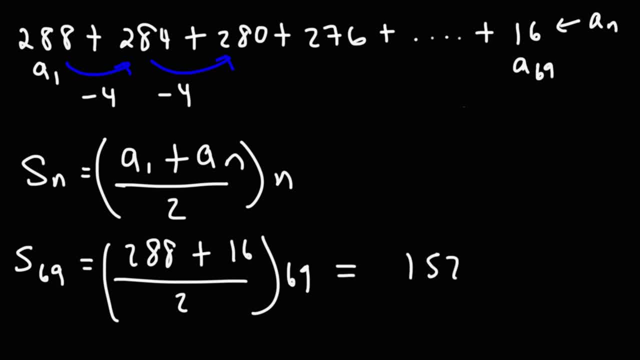 304 divided by 2 tells us that the average of all the numbers in this sequence is going to be 152, which is the average of the first and last term. 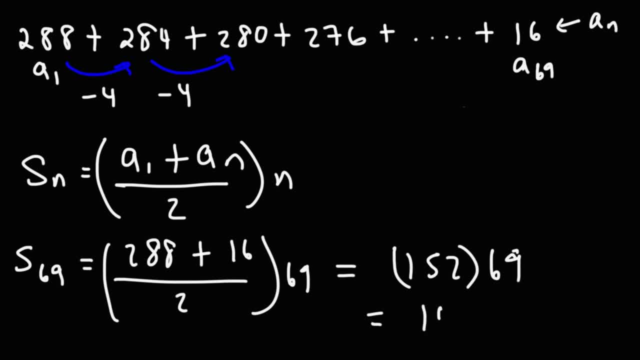 So 152 times 69 is 10,488, and so that's how you can calculate the sum of this arithmetic equation. 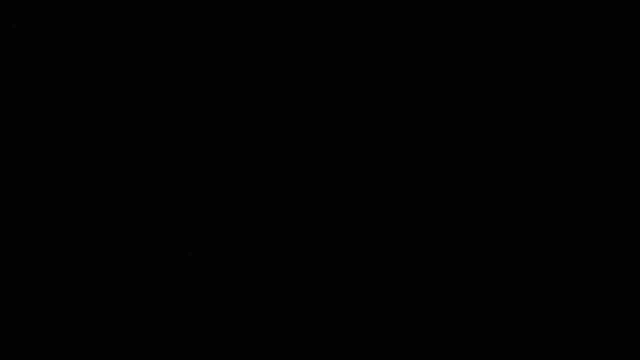 For the sake of practice, I'll give you another one. So let's say we have the numbers 96, and then 89, well let's put a plus, plus 82, plus 75, 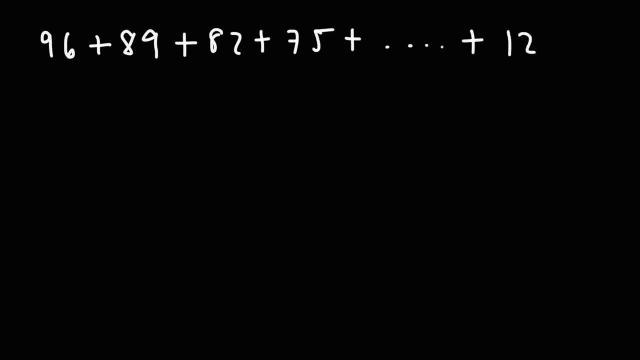 and then plus 12. Go ahead and calculate the sum of that arithmetic series. So this is the first 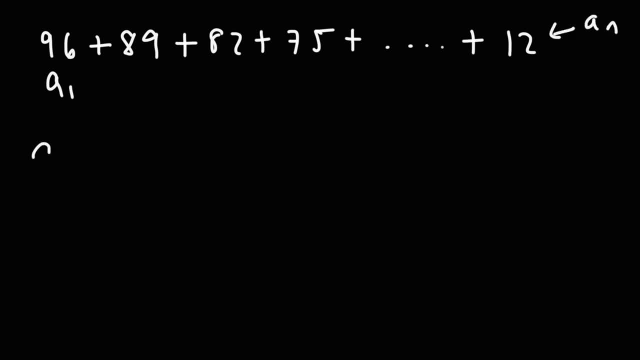 term, this is the last term. Just like before, let's calculate n, the number of terms. So a sub n is 12, a sub 1 is 96, and the common difference, so going from 96 to 89, or 89 to 96, is 96. 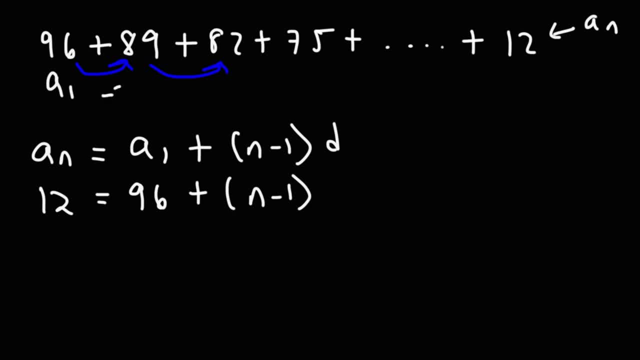 Or 89 to 82, we need to add negative 7. So d is negative 7. 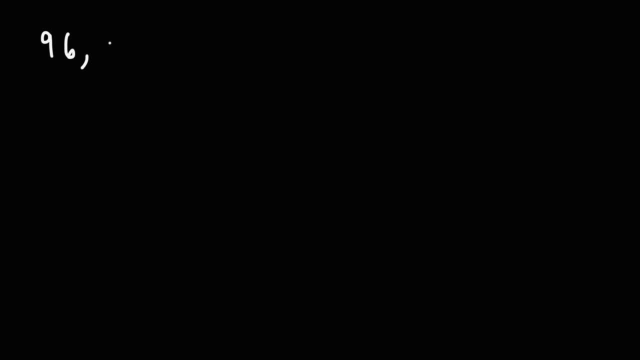 is 96 and then 89. well, let's put a plus plus 82, plus 75 and then plus 12. go ahead and calculate the sum of that arithmetic series. so this is the first term. this is the last term, just like before. let's calculate n, the number of. 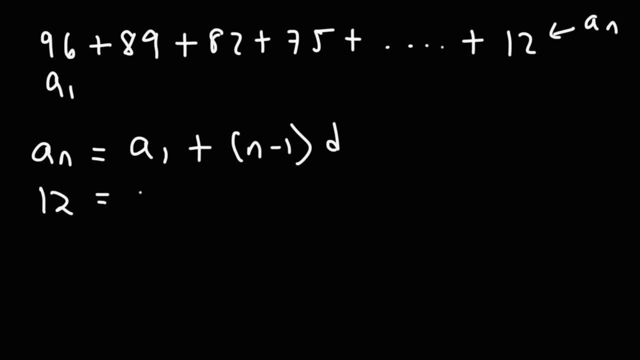 terms. so a sub n is 12, a sub 1 is 96 and the common difference. so going from 96 to 89 or 89 to 82, we need to add negative 7, so d is negative 7. that's going to give us negative 7, n plus-7 negative 1 times negative 7 is positive 7. and then we can add these two numbers: 96 plus 7 is 103. and now list: subtract both sides by 103. 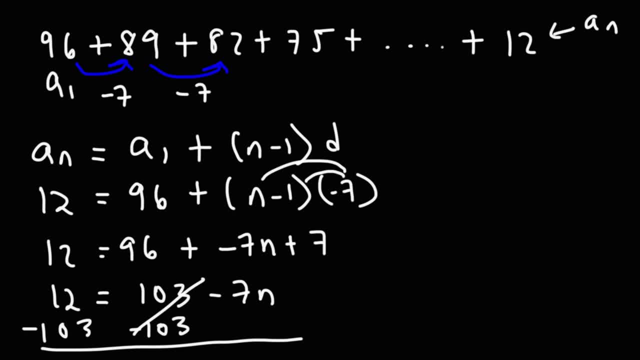 12 minus 103 is negative 2 plus 8 and the common difference e is negative. 7 plus 8 can be written as negative 7, Che e is наших third cancels as negativeaban modus 91, and then we could divide both sides by negative 7, and that is going to give. 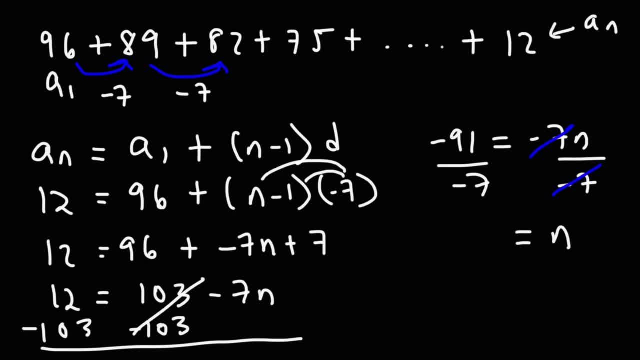 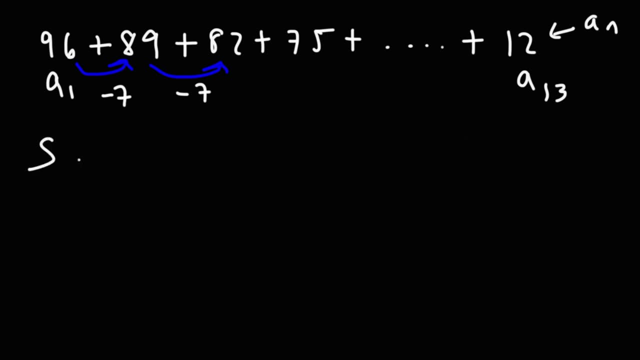 us our n value, which in this problem is 13. so 12 is the 13th term or a sub 13. so now that we have that, we can calculate the sum. so let's go ahead and let's use this formula s sub n is a sub 1 plus a sub n divided by 2 times n, so we're. 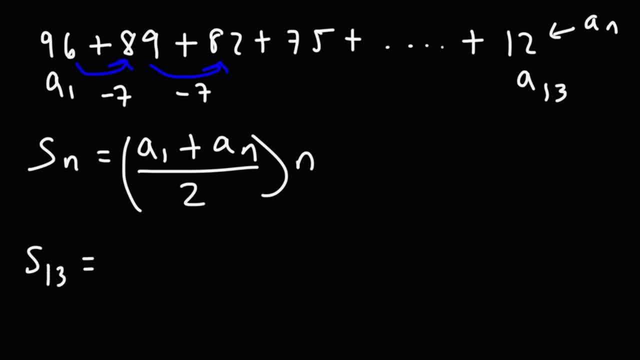 looking for the sum of the first 13 terms or the partial sum. the first term is 96, a sub n, or the 13th term is going to be 12 and n is 13. 96 plus 12 is 108. 108 divided by 2 that gives us. 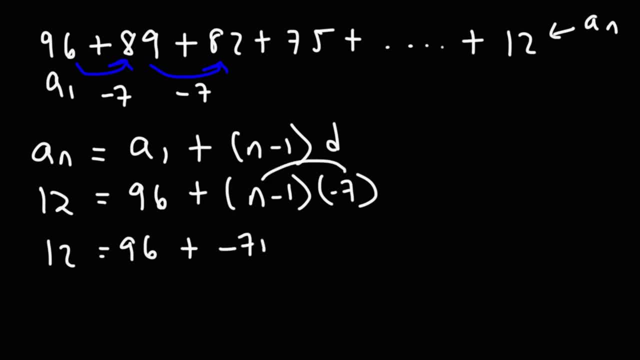 Distributing negative 7 to n minus 1, that's going to give us negative 7n plus 7. Negative 1 times negative 7 is positive 7. And then we can add these two numbers, 96 plus 7 is 103. And now let's subtract both sides. 12 minus 103 is negative 91. And then we can divide both sides by negative 7, and that is going to give us our n value, which in this problem is 13. 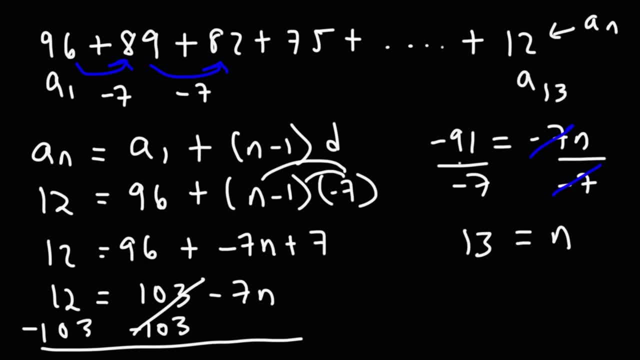 So 12 is the 13th term, or a sub 13. 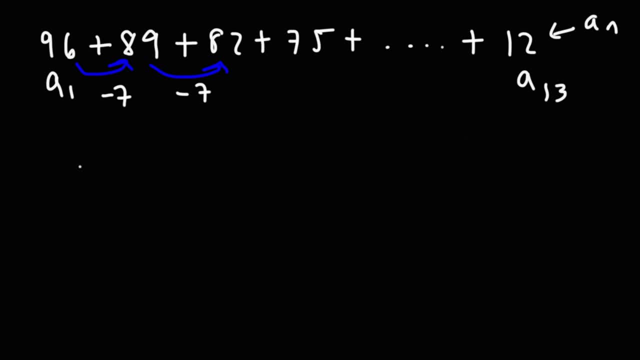 So now that we have that, we can calculate the sum. So let's go ahead and let's use this formula. S sub n is a sub 1 plus a sub n divided by 2 times n. So we're looking for the sum of the first 13 terms, or the partial sum. The first term is 96. A sub n, or the 13th term, is going to be 12. And n is 13. 96 plus 12 is 108. 108 divided by 2, that gives us 54, which is the average of the first and last terms. 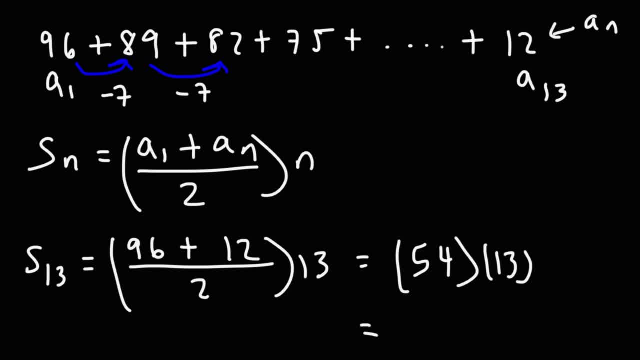 So if we take that average, 54, multiplied by the number of terms, that will give us the sum, which is 702. 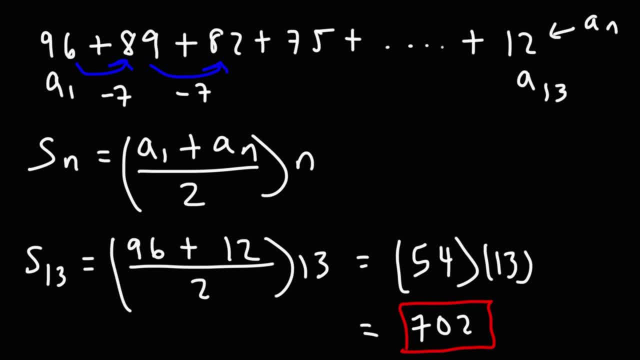 So, that's all you need to do in order to calculate the sum. And that's how you get an arithmetic sequence. Or rather, an arithmetic series. 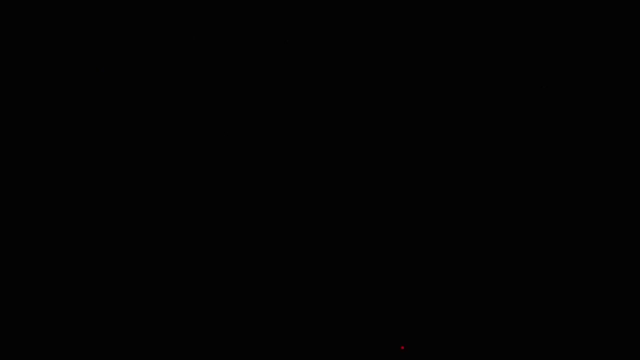 So remember, the first thing you need to do is, just to review, use this formula to calculate n, the number of terms. Once you find n, you can plug everything into this equation to get the sum of the series. 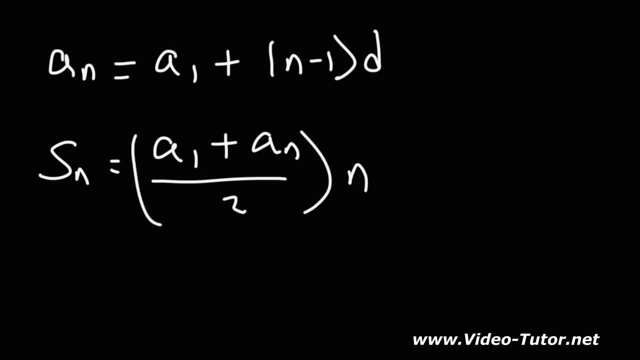 So, this is the sum of the series.